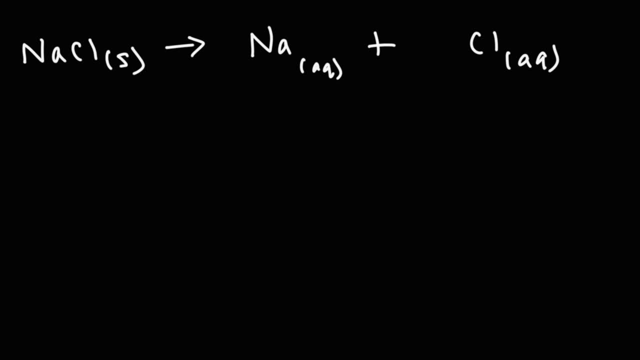 metals and alkali metals like sodium, lithium, potassium: they typically form cations with a plus one charge. The halogens, like fluorine, chlorine, bromine, iodine: they typically form ions with a negative charge. So that's all we could do for sodium chloride. Now let's move on to our next example. 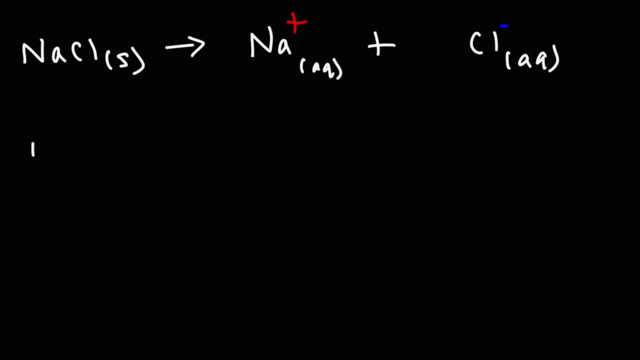 What about for ammonium bromide? Write the dissociation equation for that. Now, ammonium is a polyatomic ion. You can't break that apart, and it has a plus one charge. This is something that you need to commit to memory, So let's write the dissociation equation for that. 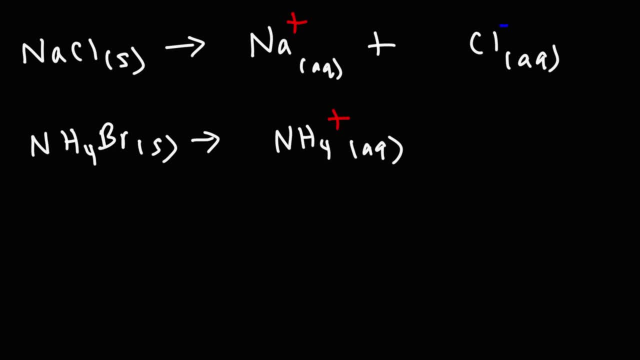 What I recommend is go to the youtube search bar, type in polyatomic ions, organic chemistry tutor, and the video should come up with a list of polyatomic ions that you need to know. So feel free to take a look at that when you get a chance. Now, bromine like chlorine- they're in the same. 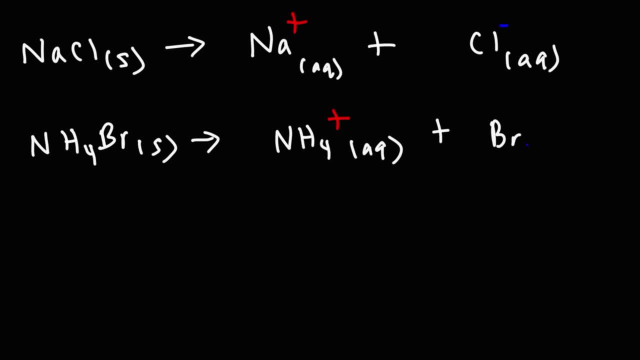 column in the periodic table. So they're going to have the same charge, That is, a one minus charge. So we're going to write the dissociation equation for that. So we're going to write the dissociation equation for that. So we're going to write the dissociation equation for that. 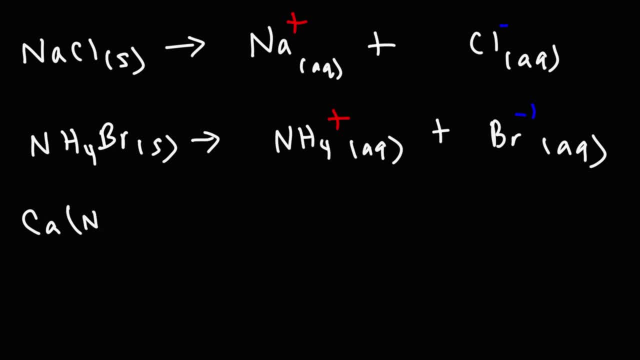 Now what about this one Calcium nitrate? Go ahead and write the dissociation equation for that And also try magnesium iodide. And also try magnesium iodide. So notice that we have one calcium ion in the aqueous phase and we have two nitrate ions. So that's going to be the coefficient for nitrate. 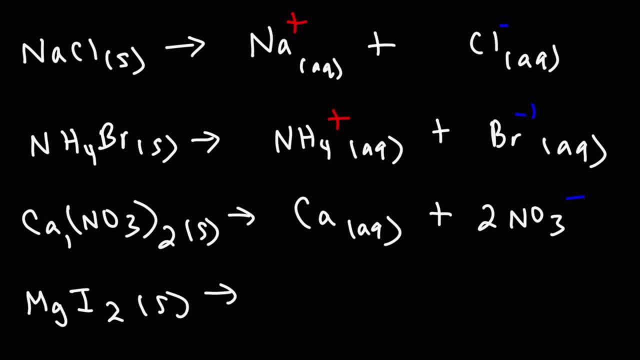 Now, nitrate is a polyatomic ion with a negative one charge. Calcium is in group two- It's an alkaline earth metal- and group two elements like calcium, strontium, barium, magnesium. they typically have a two plus charge And you can also figure this out. 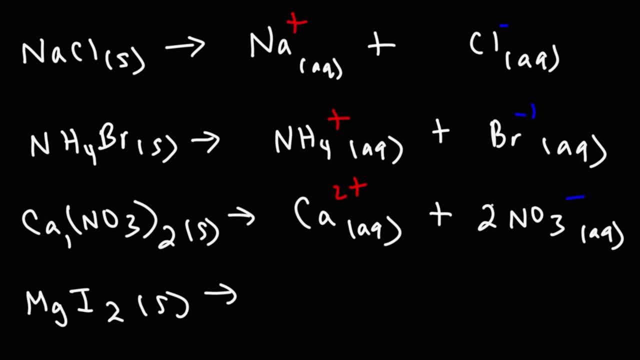 if you know the charge of the other ion, Notice that we have two nitrate ions. That's a total charge of negative two. In order to balance that, calcium has to have a two plus charge so that overall the total charge on the right side is zero. 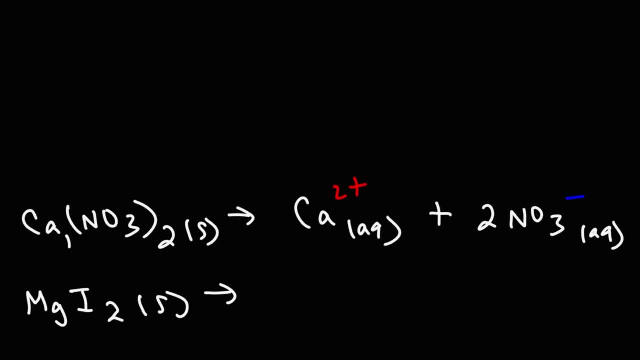 So if you wanted to calculate the charge on calcium, here's what you can do. In calcium nitrate, we have one calcium ion and we have two nitrate ions. The net charge is going to be zero. Now, nitrate has a charge of negative one, so we can replace it with negative one. 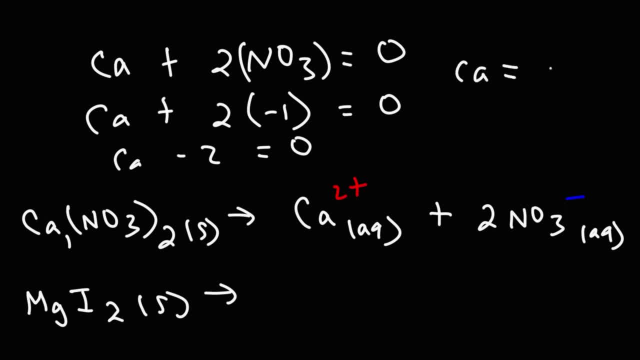 Solving for calcium. if we add two to both sides, we get that calcium is going to have a plus two oxidation state or two plus charge, So you can actually solve for it. if you don't know what the charge is Now for magnesium: iodide magnesium is an alkaline earth metal, just like calcium. 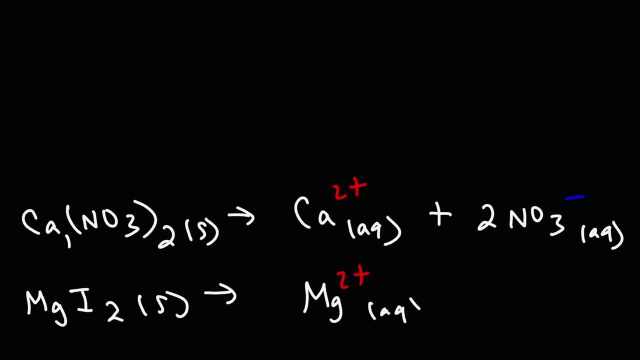 so it's going to have a two plus charge. Iodide, there's two of them. We can see the subscript two. Like the other- halogens, chloride and bromide- it's going to have a negative charge, And so that's how we can write the dissociation. 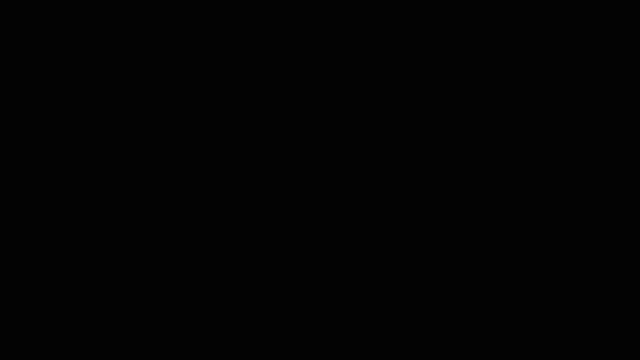 So we're going to write the dissociation equation for magnesium iodide. Go ahead and try these: Calcium chloride, sodium carbonate, potassium phosphate and barium hydroxide And barium hydroxide And barium hydroxide. 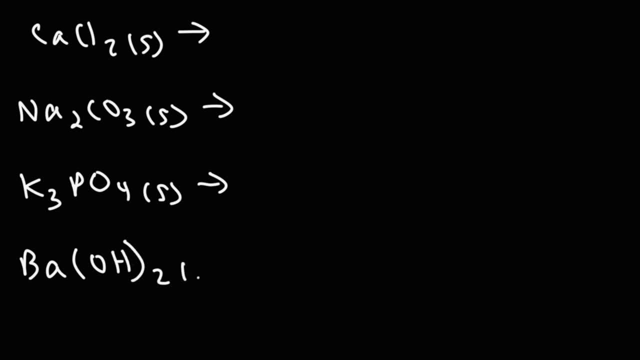 Write the dissociation equation for each of the following ionic compounds. Alright, let's start with the first one. We have calcium chloride. We know calcium is in group two, It's going to have a two plus charge and we have two chlorine ions, so the coefficient will be two and we know chloride has a negative. 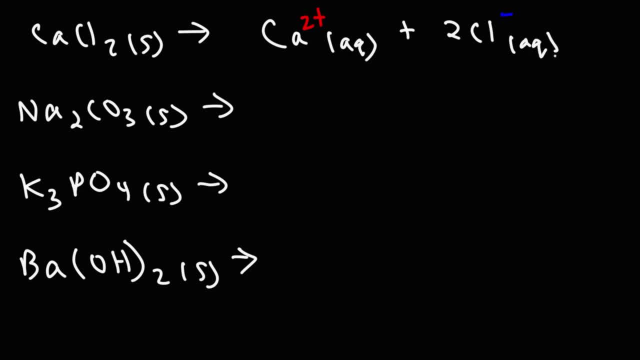 charge and we'll put the phase aqueous, which means it's dissolved in water. Now, moving on to the next one, we have sodium carbonate. Notice that we have two sodium ions. The subscript is two, so that's going to become the coefficient. Sodium is an alkali metal found in group one. 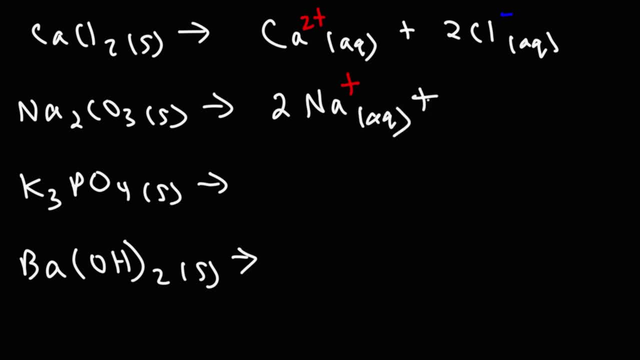 so it's going to have a plus one charge: Carbonate. what is the charge on carbonate? Notice that we only have one carbonate as a whole. It's a polyatomic ion. Now, sodium has a plus one charge. There's two of them, so that's a total charge of two plus. 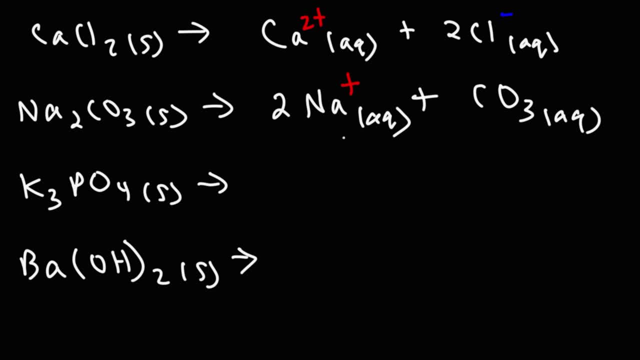 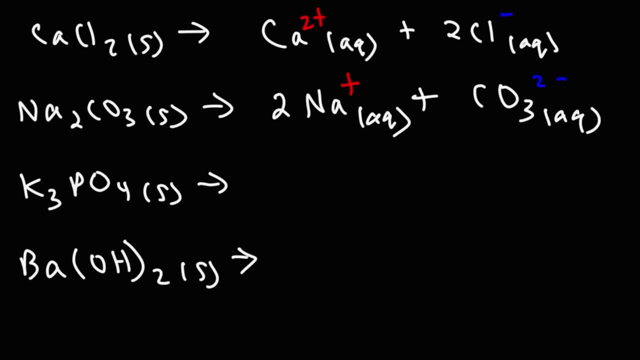 you're just going to know what the charge is. Now, moving on to potassium phosphate, Notice that we have three potassium atoms, or rather three potassium ions. Potassium is an alkali metal, just like sodium, so it's going to have a plus charge. Now, what about PO4, phosphate? 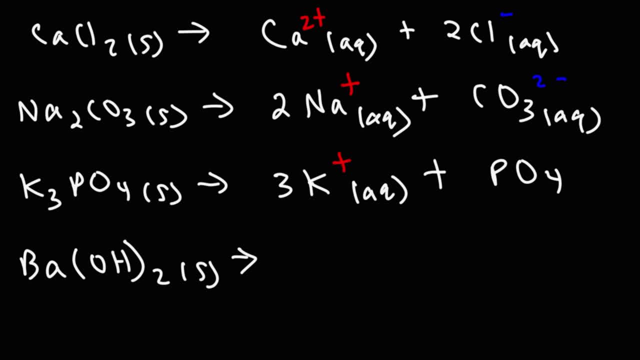 another polyatomic ion. What's the charge on that? Potassium has a plus one charge times three, that's plus three. We only have one phosphate. so to neutralize that three plus charge we need a three minus charge. So it's phosphate three minus. 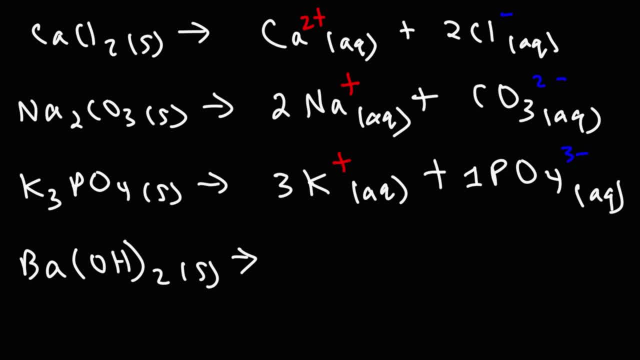 Now what about the last one, barium hydroxide? Barium, like calcium, is an alkaline earth metal. Because they're in the same group in the periodic table, they will have the same charge as an ion, in this case a two plus charge. 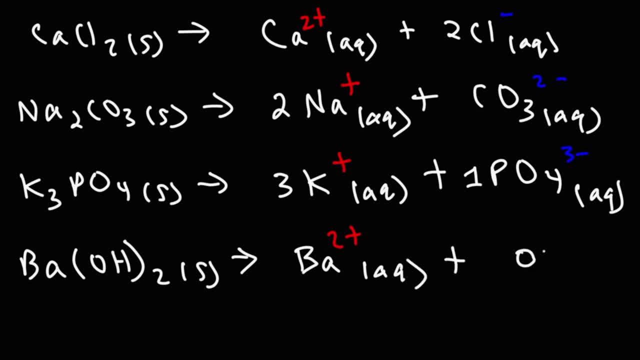 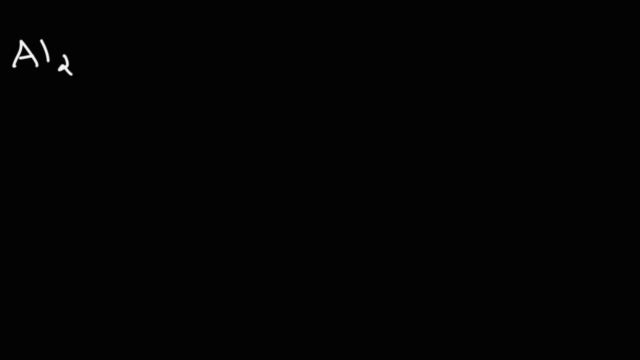 Next we have another polyatomic ion hydroxide and notice that we have two of them Now hydroxide. this is one of those things you need to know. it has a negative one charge. so that's it for those four examples. try this one: aluminum sulfate, al2, so43. go ahead and write. 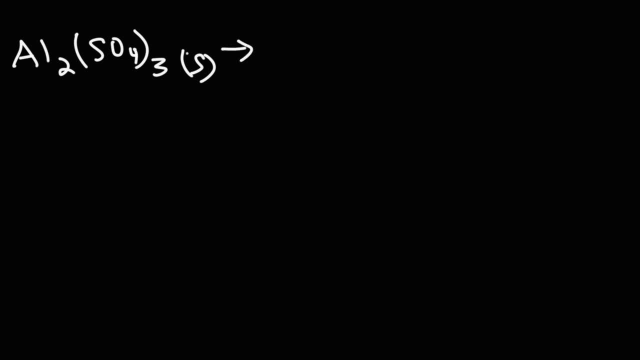 the dissociation equation for that. so we have a subscript of two, which means we have two aluminum cations, and we have a three in front of so4, which means we have three sulfate ions. now aluminum, it's in group 3a of the periodic table, which means that it's going to have a 3. 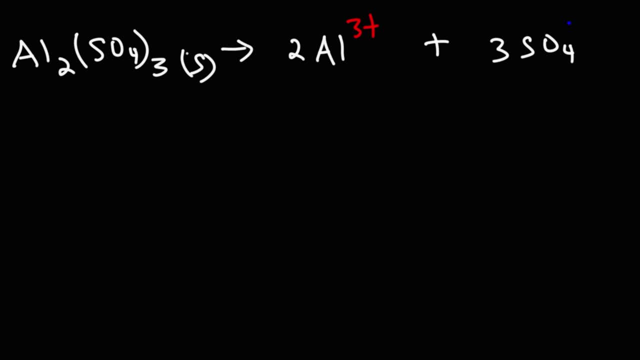 plus charge. sulfate is a polytomic ion with a 2 minus charge, and that's all we need to do for that one. now let's try one more example: m3po4. now M is some unknown metal, it's an unnamed metal, but nevertheless we want. 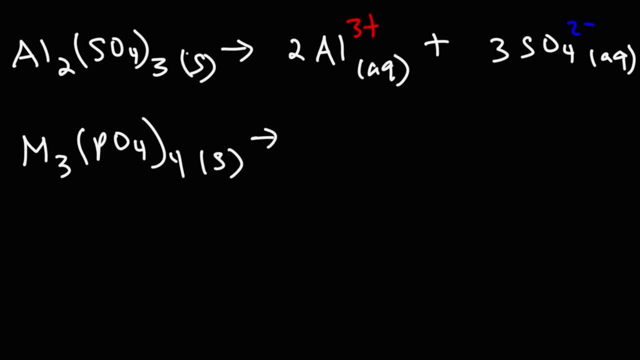 to write the dissociation equation for this ionic compound. so we have three of this unknown metal ion. we don't know the charge, so we're going to figure that out. we have four phosphate ions. we do know the charge on phosphate: it's three minus. we've covered it already. but the question is what is the missing charge? 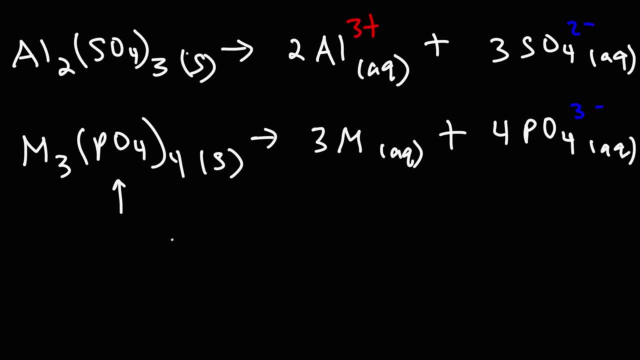 on the metal ion. let's write an equation to find out. so we have three of the metal ions and we have four phosphate ions. the net charge has to be zero for this neutral ionic compound. now what we're going to do is we're going to 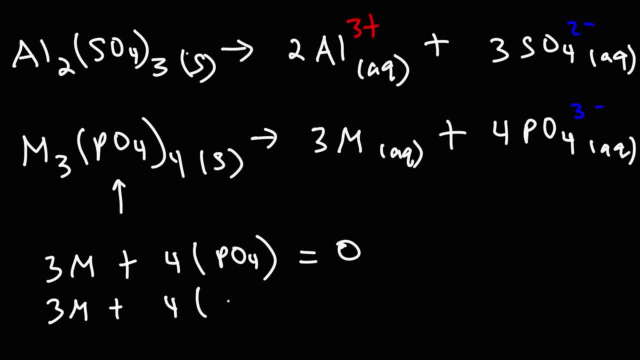 replace the phosphate with its charge. phosphate has a negative 3 charge. now 4 times negative 3 is negative 12. so we have 3m minus 12 is equal to 0. next we're going to add 12 to both sides, so we get 3m is equal to 12, and then we'll 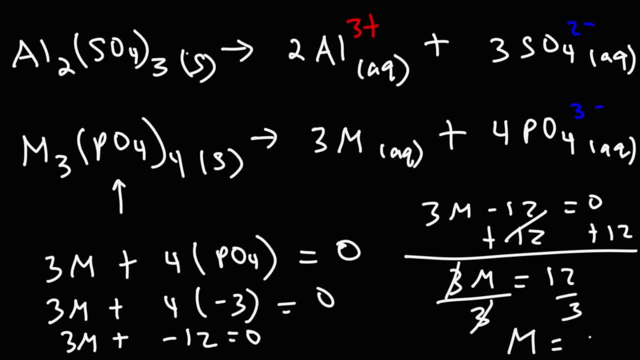 divide by 3. so this tells us that the metal has a plus 4, or rather a 4 plus charge. so if you know the charge on one ion, you could find the charge on the other ion by writing an equation. you need to set the equation equal to zero because overall, the ionic compound is neutral.